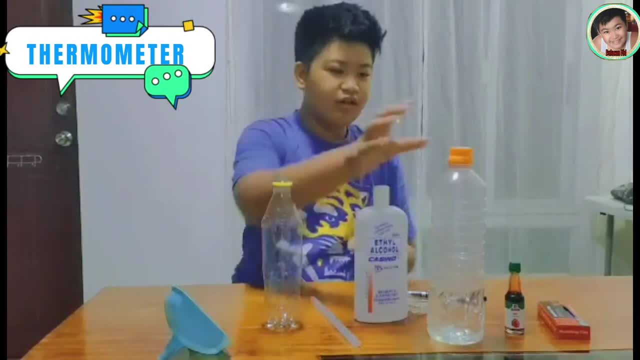 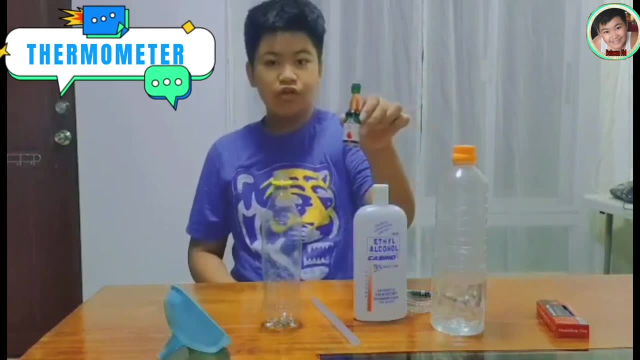 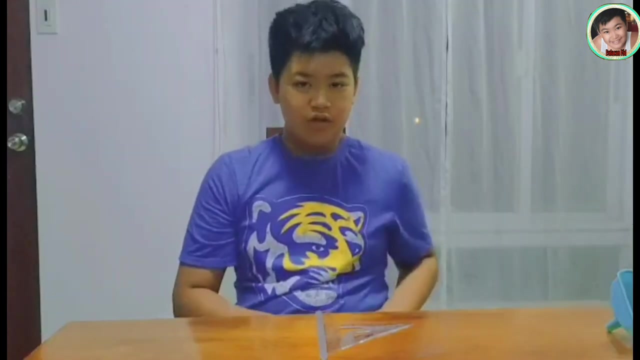 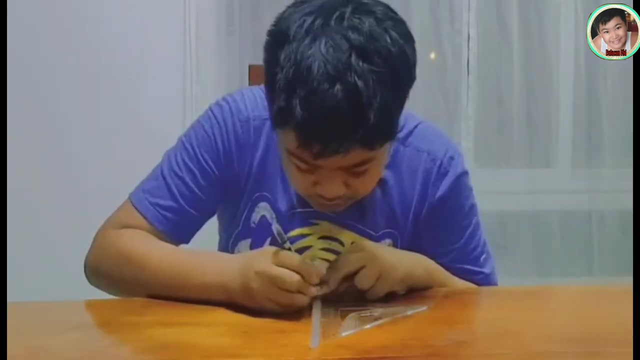 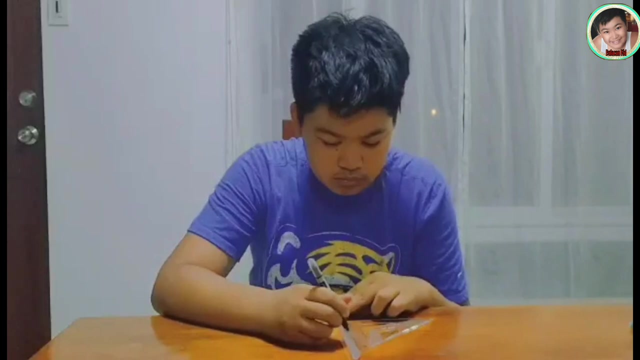 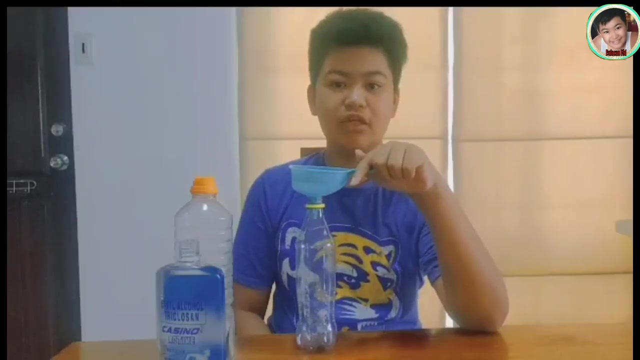 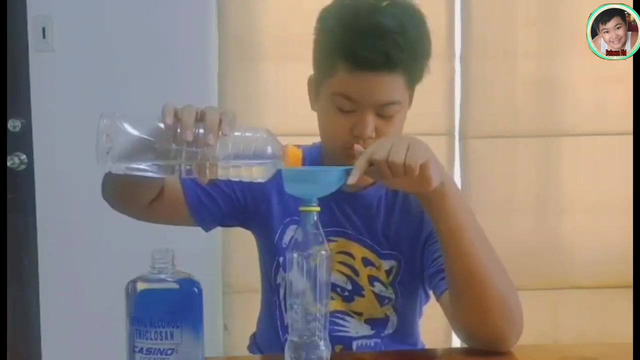 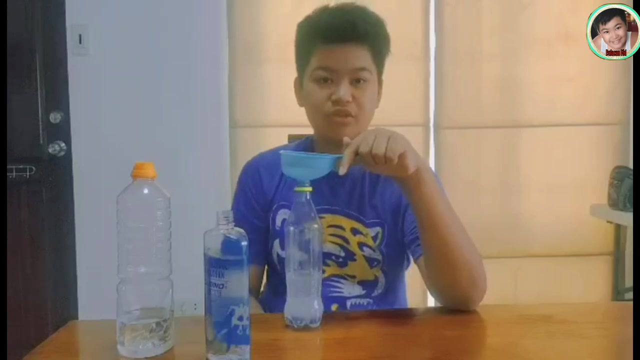 of rubbing alcohol and water, food coloring and clay. Now to start off, we're going to mark the straw in equal increments. This will help to tell the temperature later on. Next, put equal parts of water and rubbing alcohol into the bottle, Add a few drops of food coloring and mix. 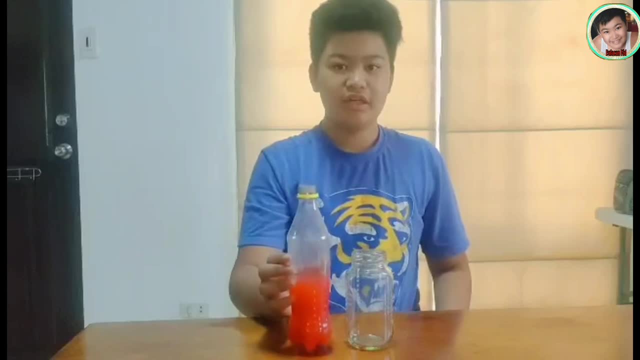 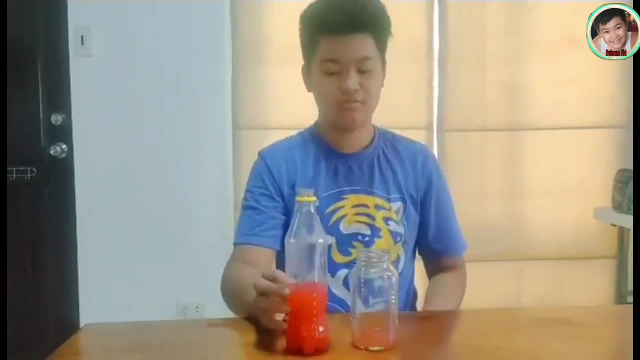 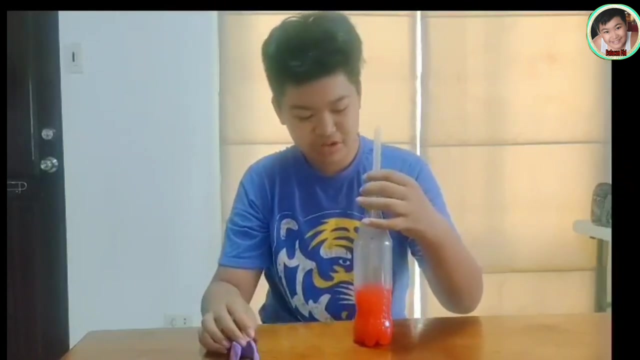 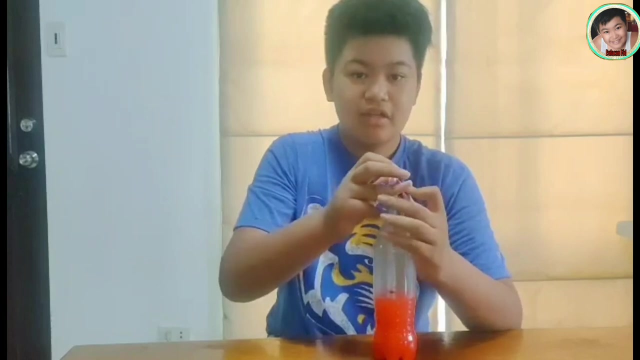 Now you want to take a little of this solution to save for later on. Then you want to insert this straw into the bottle, making sure the lower portion is fully submerged, Then add clay at the top to make it airtight, And with some of that extra mixture you'll be able. 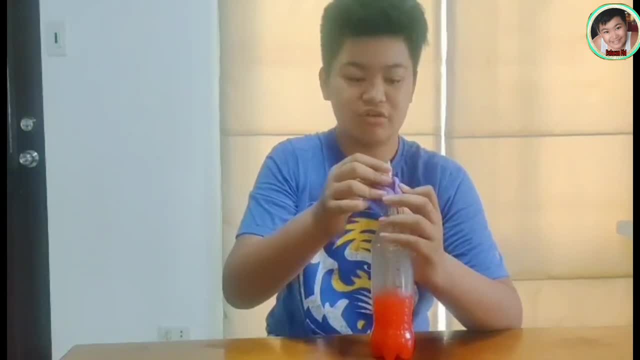 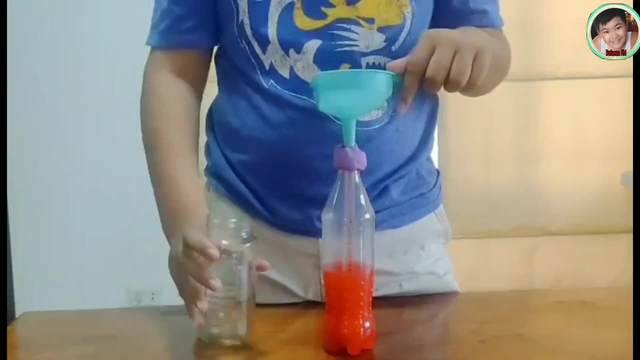 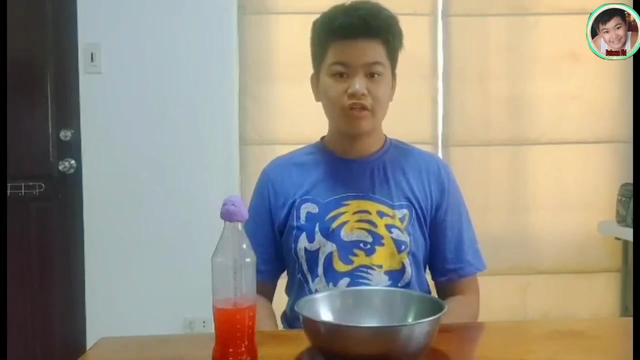 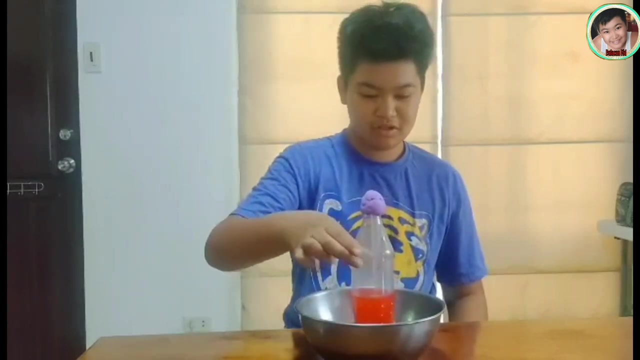 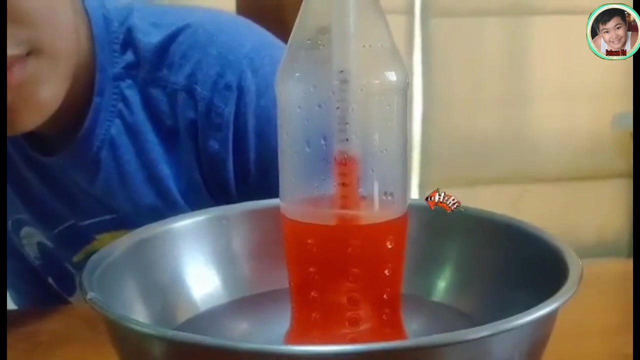 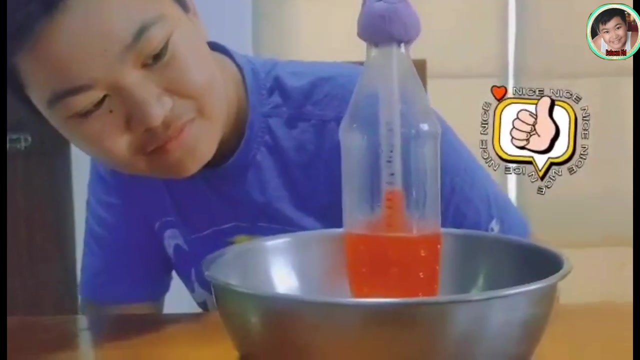 to fill the straw with the mixture you saved. Pour that back into the straw to fill it part way up. Now you're ready to use your thermometer. If you place it in warm water, the liquid in the straw will dry. oh, it's working. it's working, it's going up and it will also drop when placed in. 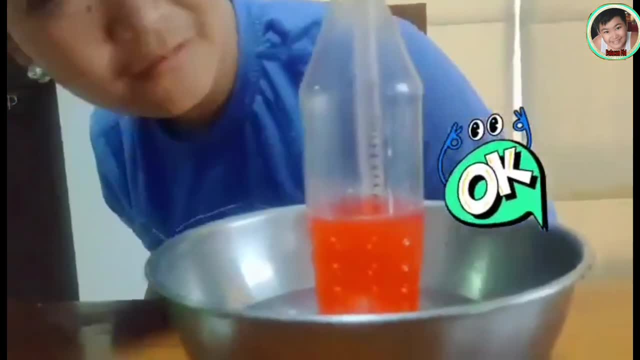 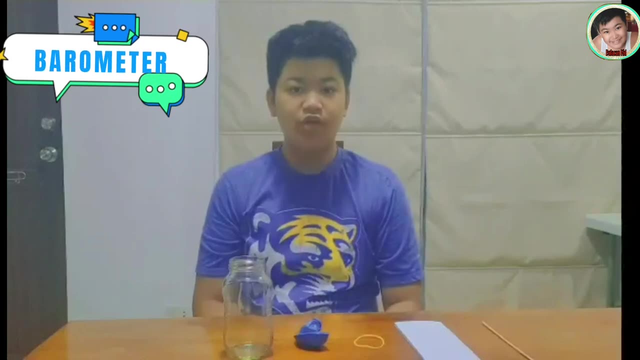 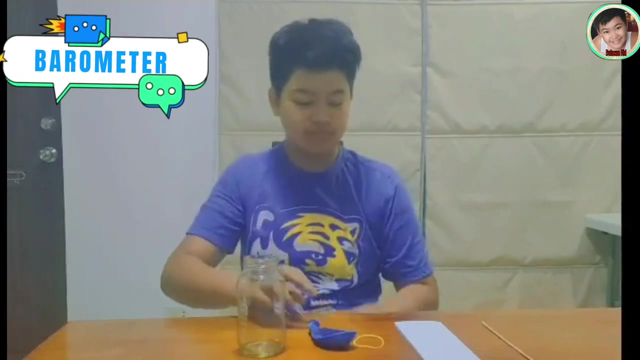 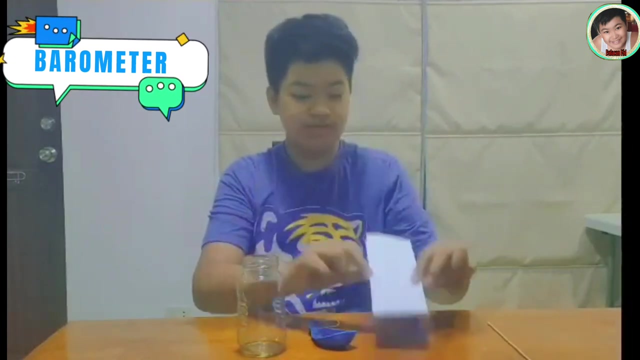 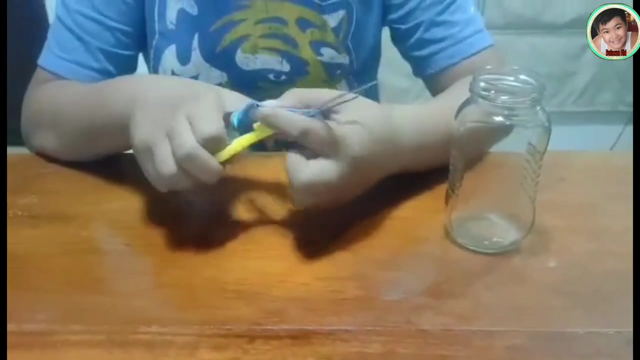 cool water. oh wow, it's going down for the barometer. you'll need a glass jar, a balloon, rubber bands, a large index card and a bamboo skewer. first cut the neck off the balloon and stretch it around the top of the glass jar. it should be.